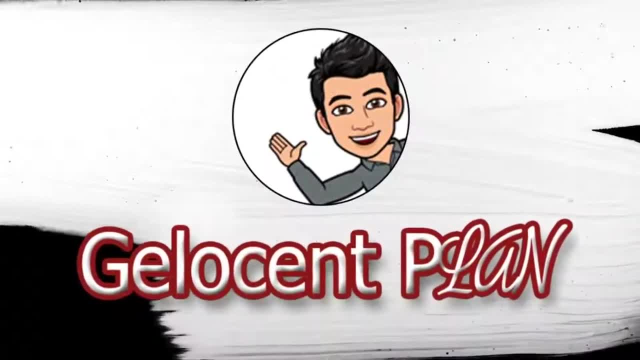 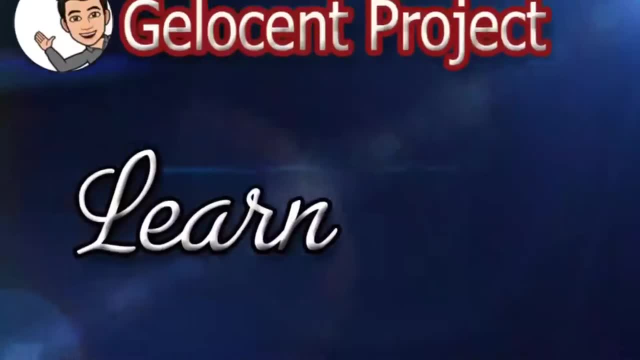 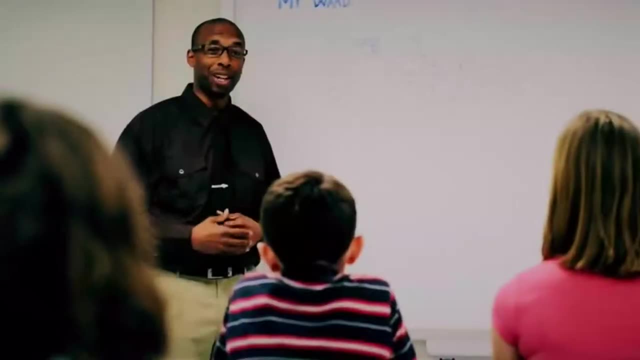 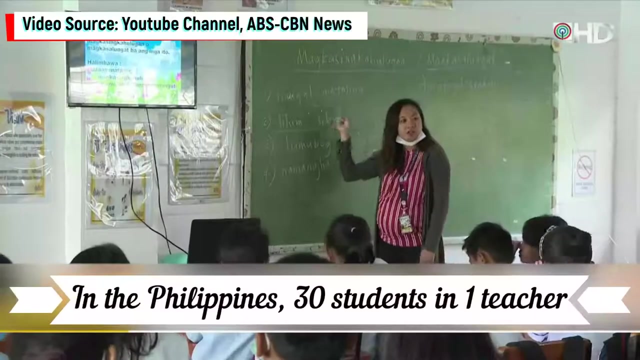 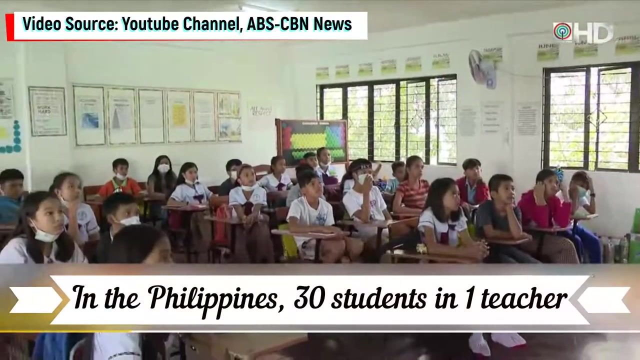 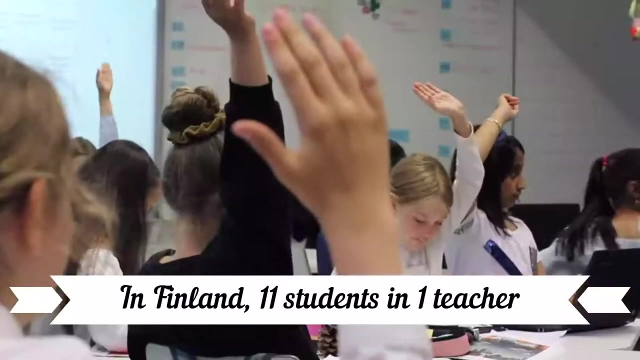 Teachers and doctors both play an essential role in our life. In the year 2018, did you know that in the Philippines, for every 30 students, there is only one teacher? In Finland, for every 11 students, there is one teacher. 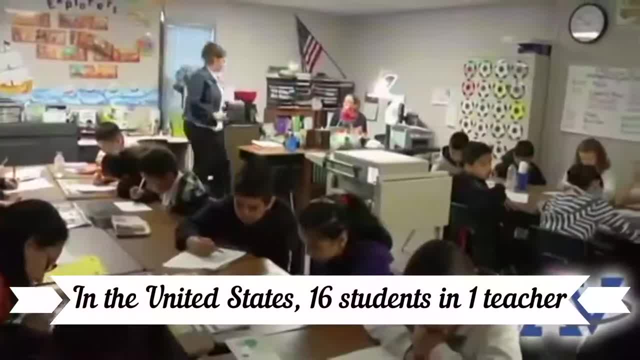 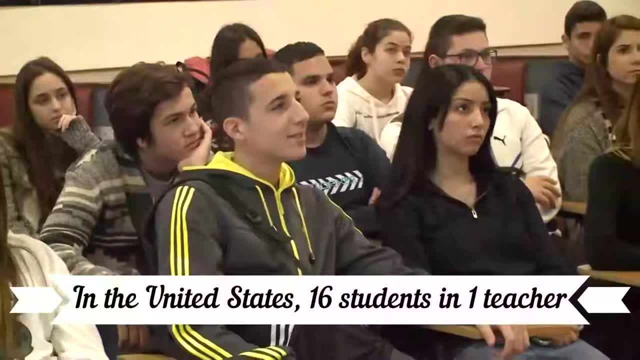 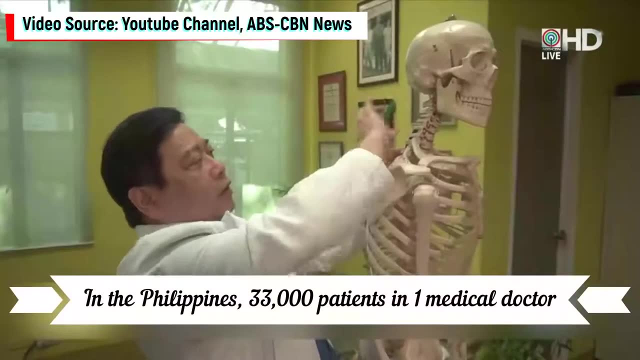 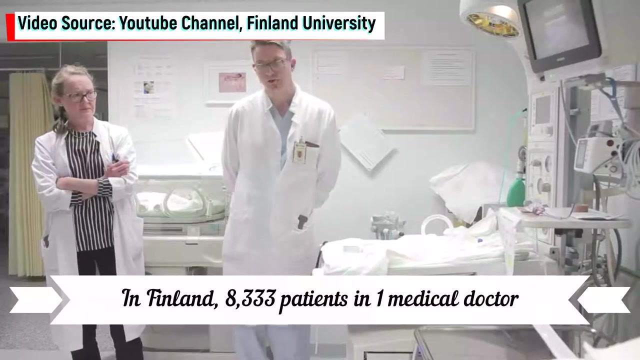 In the United States, for every 16 students, there is one teacher In the year 2016,. did you know that in the Philippines, for every 33,000 patients, there is only one medical doctor? In Finland, for every 8,333 patients, there is only one medical doctor. 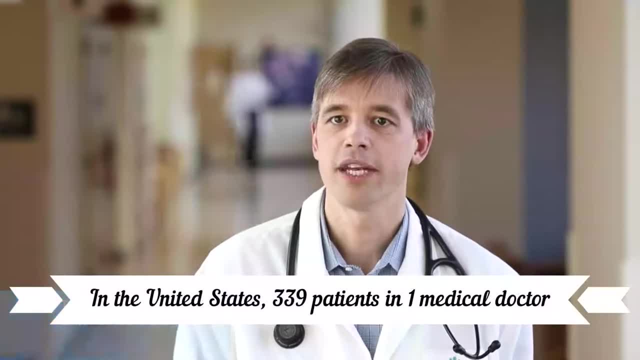 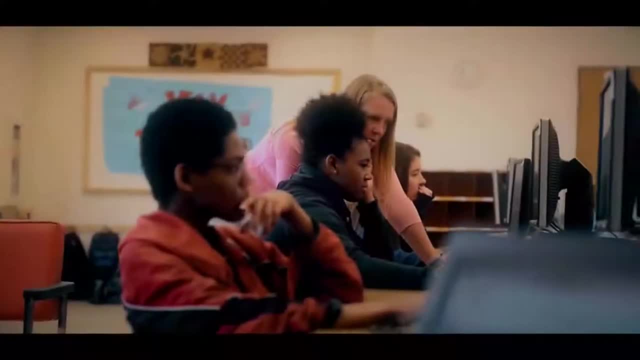 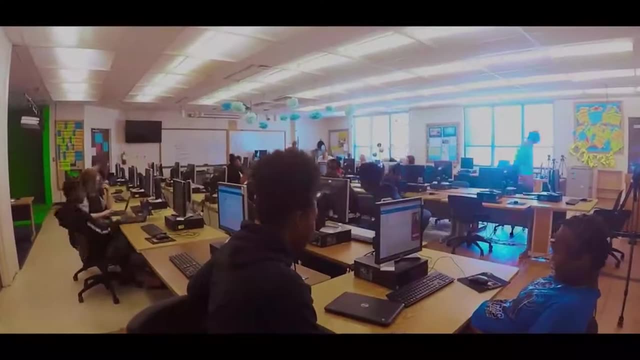 In the United States, for every 339 patients, there is only one medical doctor. In the United States, for every 8,333 patients, there is only one medical doctor. What mathematical concept explained this? These are some of the real-world facts about ratio. 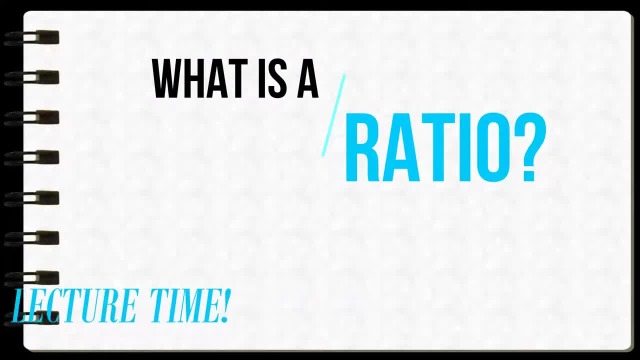 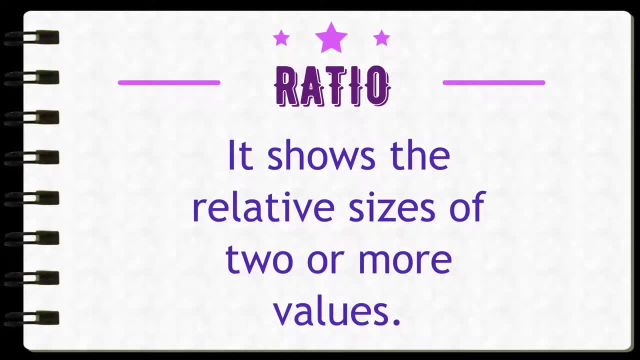 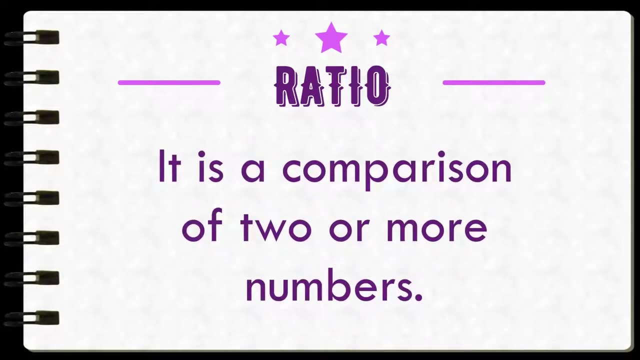 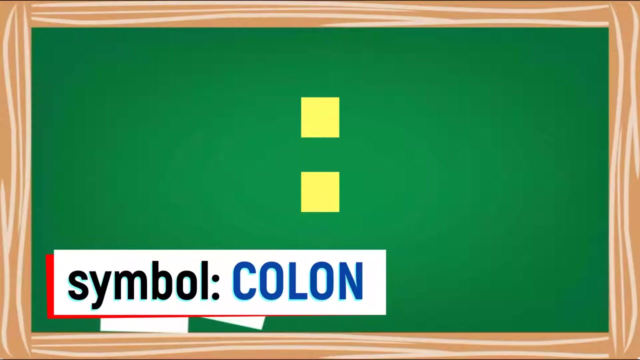 So what is a ratio? A ratio shows the relative sizes. A ratio shows the relative sizes of two or more values. In other words, it is a comparison of two or more numbers. Let's take a look at this symbol. This symbol is a column. It is the usual and most common symbol to indicate ratio. 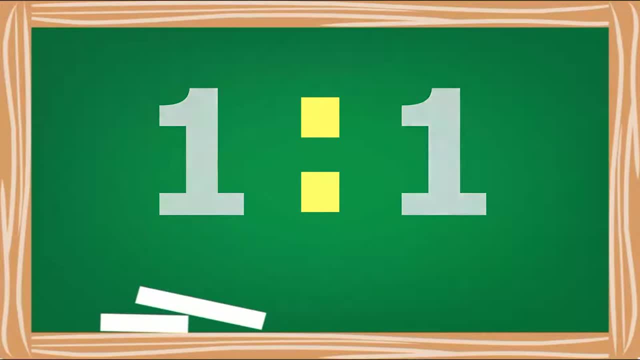 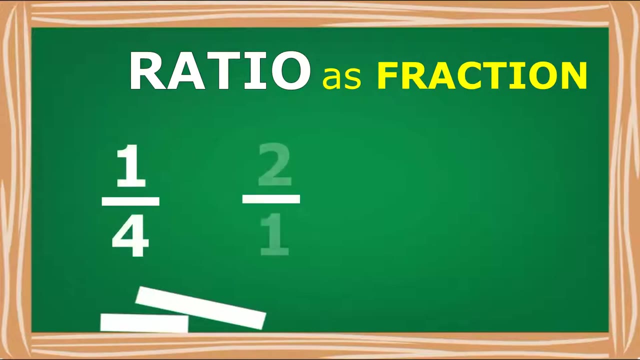 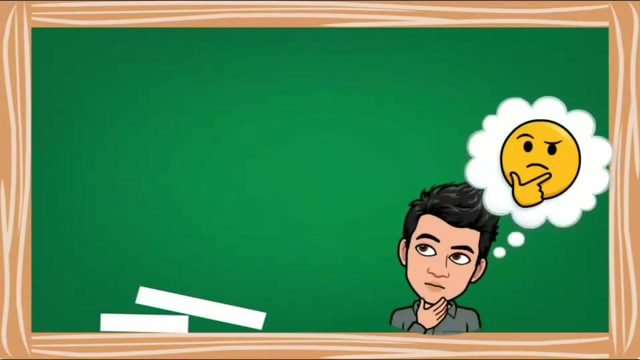 Now here is an example of a ratio: 1 to 1, 1 to 3. However, most of the application of ratio is expressed in fraction form, like one-fourth, two-one, five-thirds. So just like fractions, ratios must be simplified all the times. 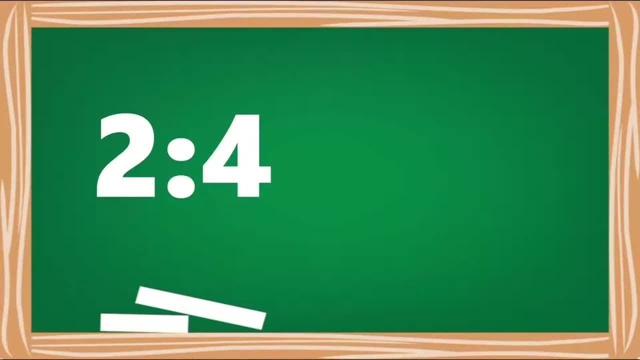 So let's write each ratio in simplest form. Both numbers can be divided by 2, so this ratio can be written as 1 to 2.. Both numbers can be divided by 5.. This ratio can be simplified as 1 to 5.. 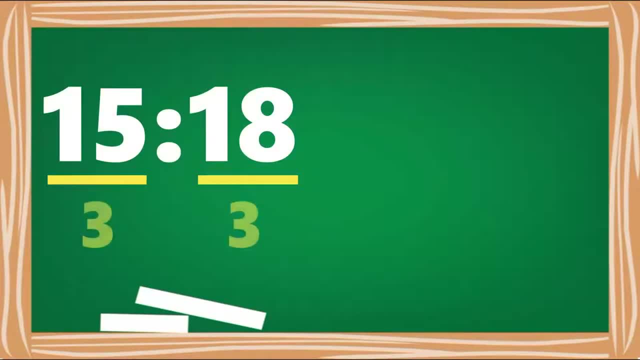 Both numbers can be divided by 3, so this ratio can be simplified to 5 to 6.. Try this. You can pause the video to check it out. The correct answer is 2 to 5 to 7.. The correct answer is 2 to 5 to 7.. 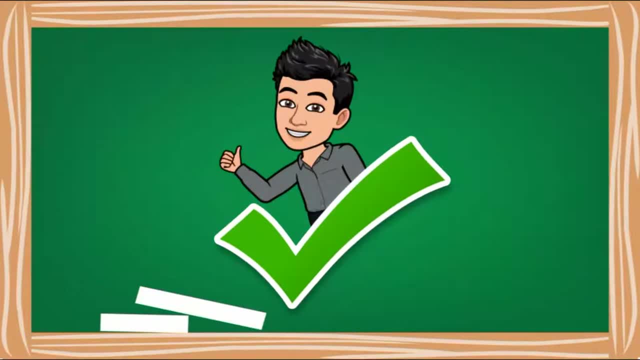 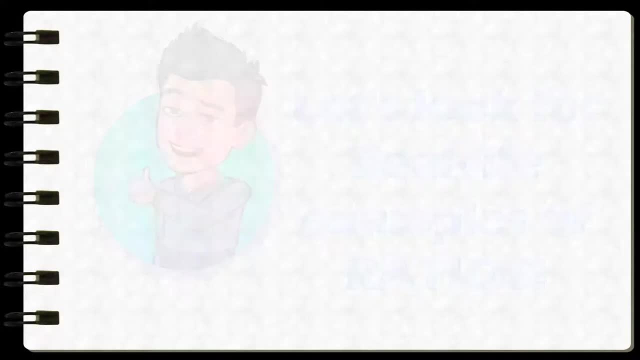 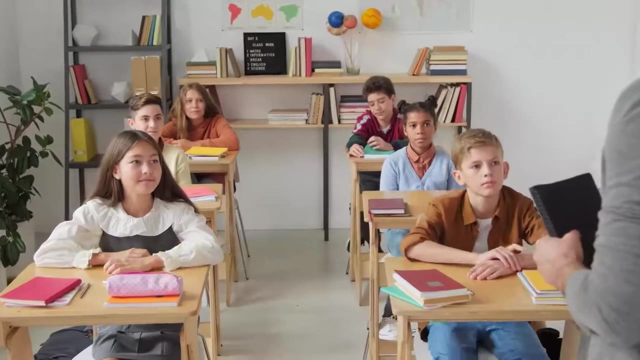 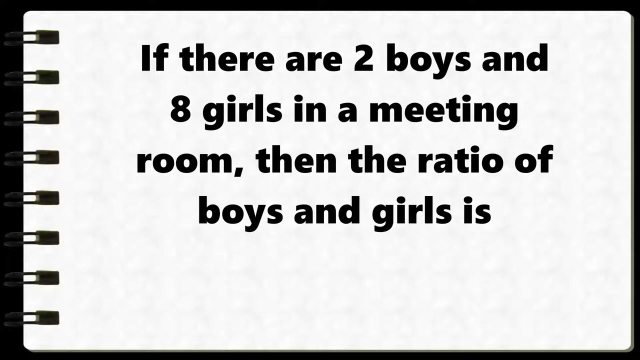 These examples are also called equivalent ratios. Very easy, right Now let's write situations into ratios. Boys and girls. If there are two boys and eight girls in a meeting room, then the ratio of boys and girls is 1 to 4.. 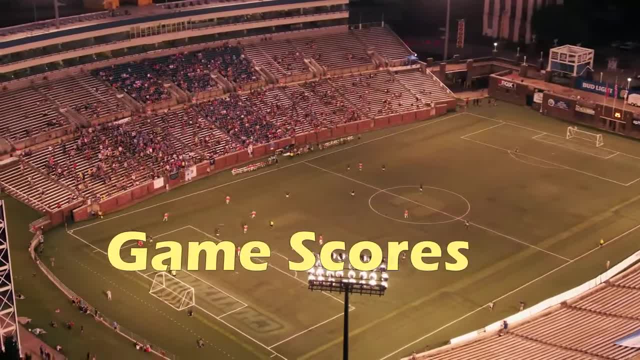 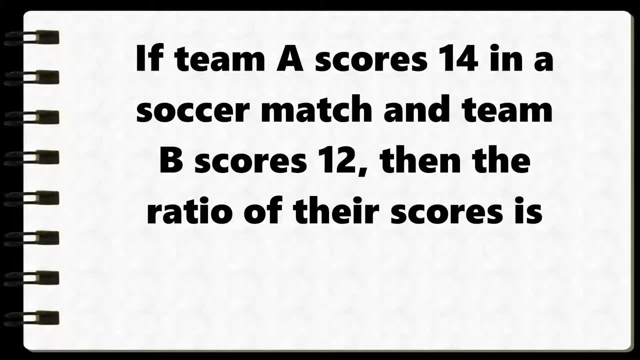 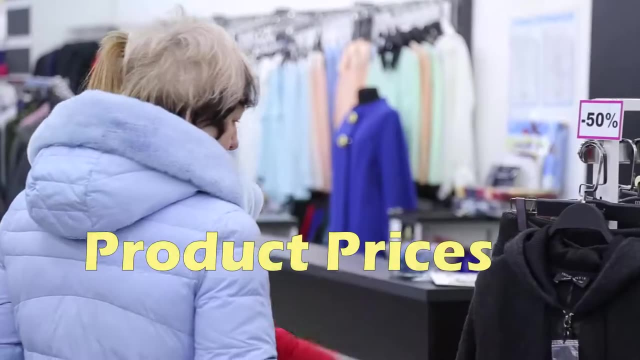 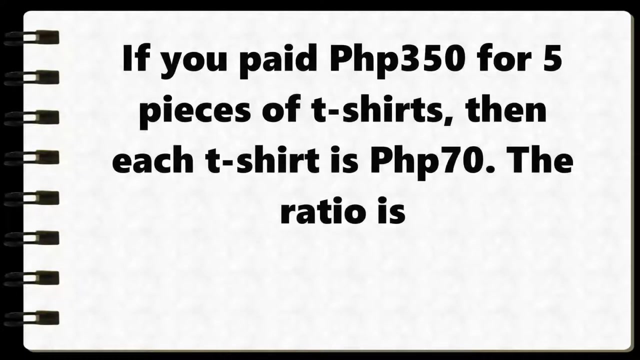 Game scores: If team A scores 14 in a soccer match and team B scores 12, then the ratio of their scores is 7 to 6.. Product prices: If you pay 350 pesos for 5 pieces of t-shirts, then each t-shirt is 70 pesos. 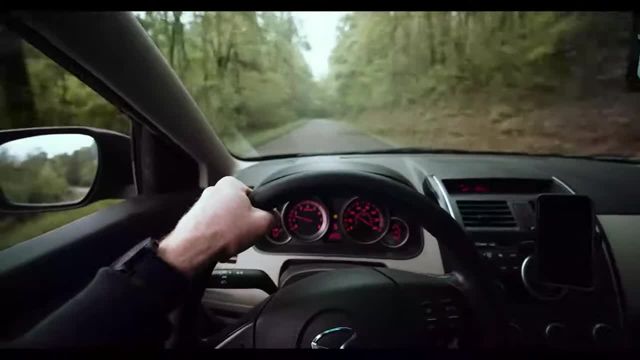 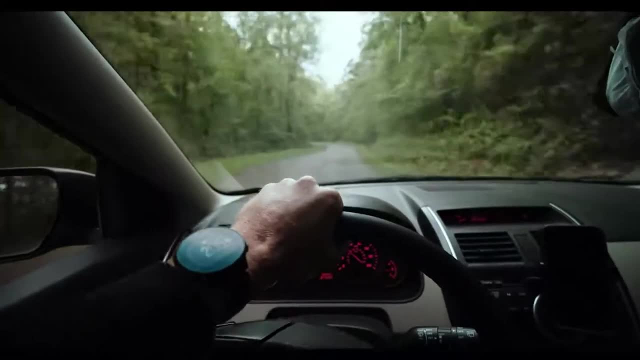 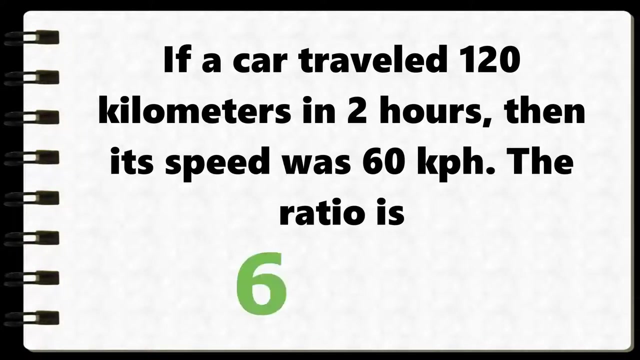 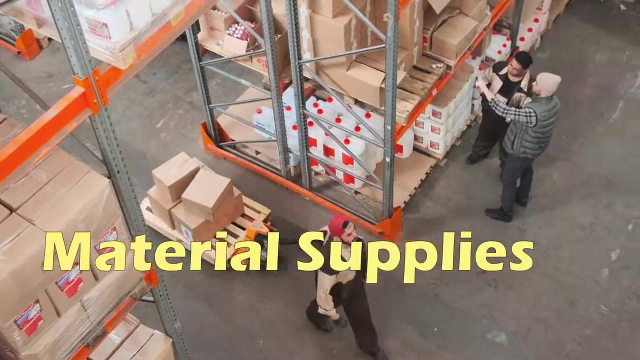 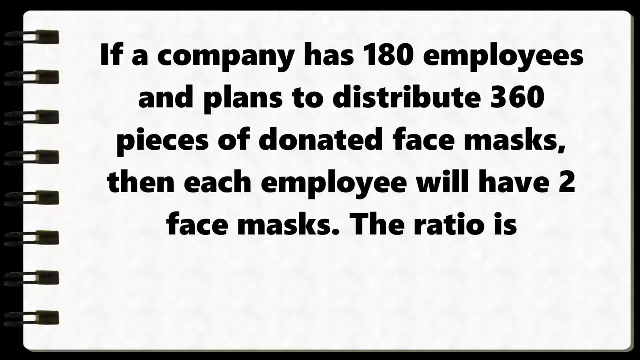 The ratio is 70 to 1. Car speed: If a car traveled 120 kilometers in 2 hours, then its speed was 60 kilometers per hour. The ratio 60 to 1.. Material supplies: If a company has 180 employees and plans to distribute 360 pieces of donated face masks, 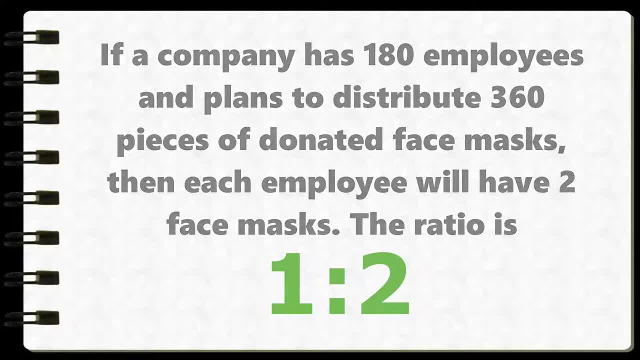 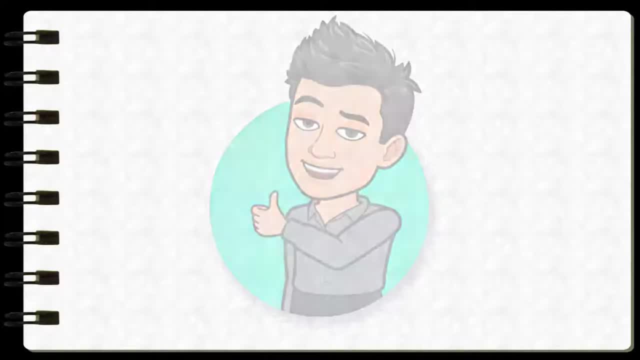 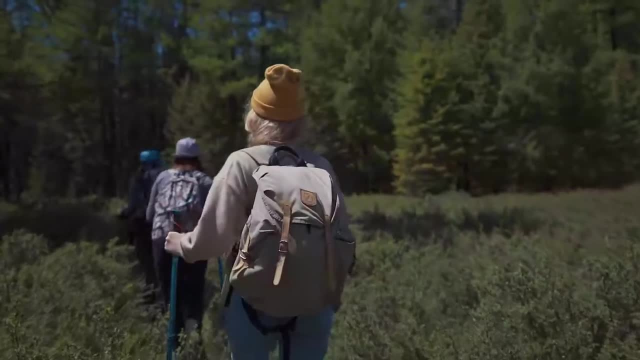 then each employee will have two face masks. The ratio 1 to 2.. That's it. There are many real-life examples of ratios. As you can see, The ratio is 1 to 2.. Whatever you do, wherever you go,